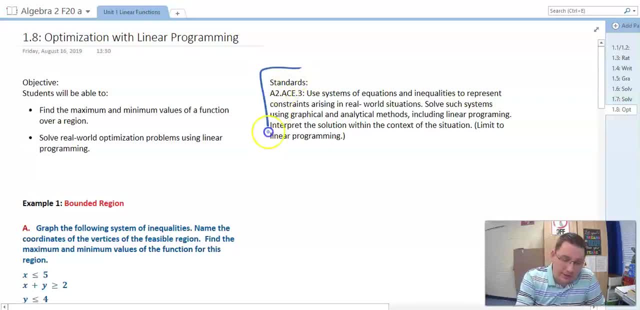 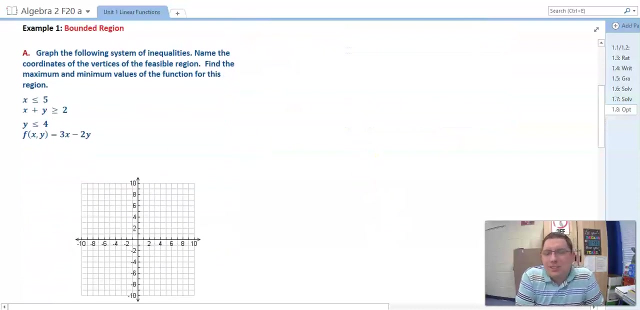 using linear programming. And this finalizes what we've been looking at in the last few sections in ACE.3, as we look at using systems of equations and inequalities to represent constraints in the real world and then solve such systems to include linear programming. And that's what we're looking at today. So let's look at example 1.. We call this a bounded. 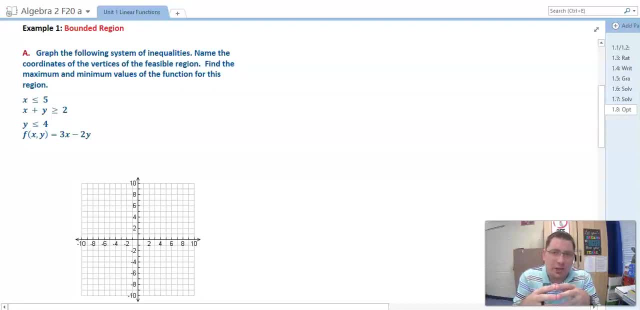 region because, like the examples we saw in 1.7, we're going to see that these different shades are going to overlap and make like a triangle or a pentagon or some type of shape where the shades stay in the same area in the end. So let's look at this problem here. 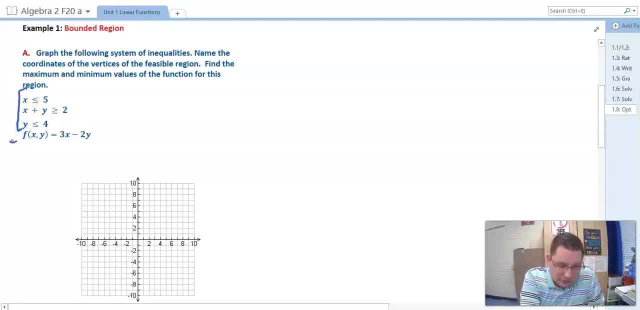 So we've got three inequalities and this is what we're going to pay attention to, and we'll get to this little piece afterwards and I'll show you how that works. So grab the following system of inequalities: name the coordinates of the vertices of the feasible. 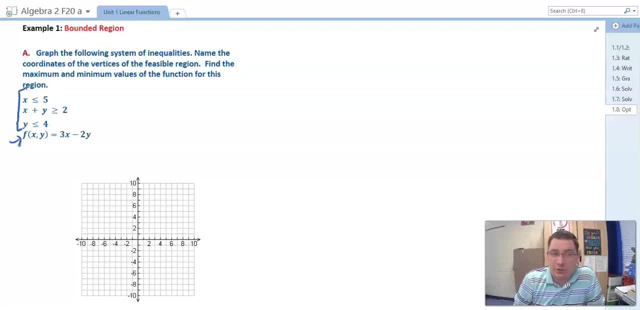 region and then find the maximum and minimum values for this region. So I've got three inequalities that we're going to look at. So I'm going to do the first one in red, I'll do the second one in orange and I'll do the third one in blue, So we can see the different. 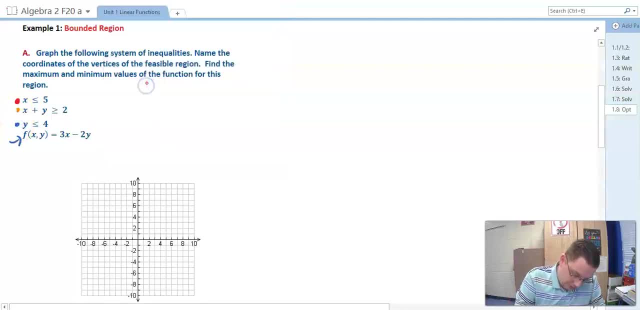 pieces and how they work. So, starting with the one in red, we've got: x is less than or equal to 5.. So x is 5 and that's equal to. so I'm going to do a solid line. and it's less than. so this shading will. 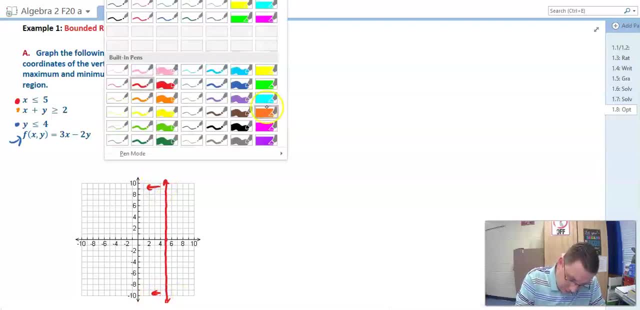 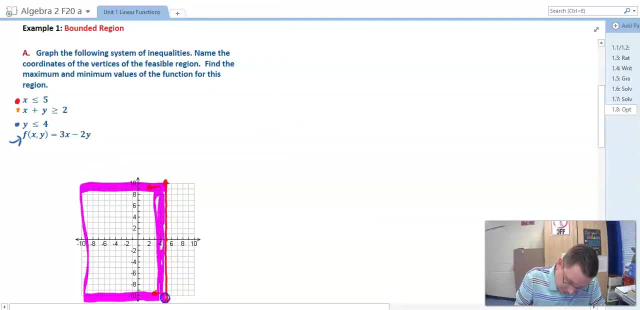 be to the left Now. you could do your highlights if you want to, and so I can come in here with a little bit of pink, and so all my pink would be all of this region. Again, I'm going to make sure you're as close to this line as possible so you can see where the overlap. 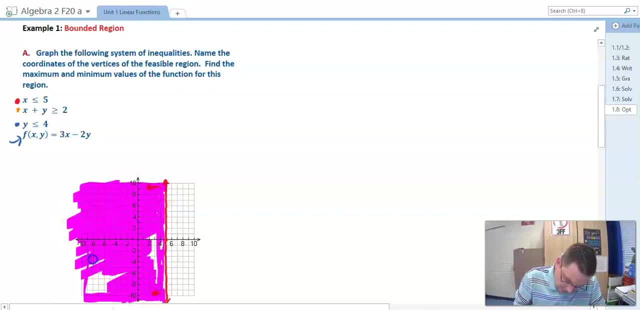 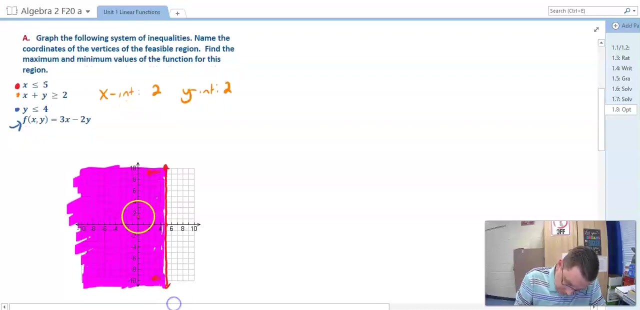 will be. So the second line, x plus y, is greater than or equal to 2, that's in standard form. So my x intercept is going to be 2, my y intercept is going to be 2.. So that is here and here. 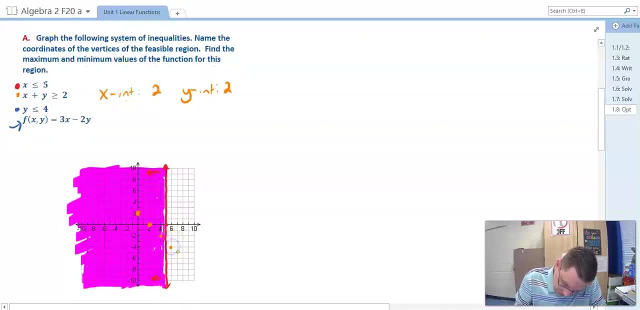 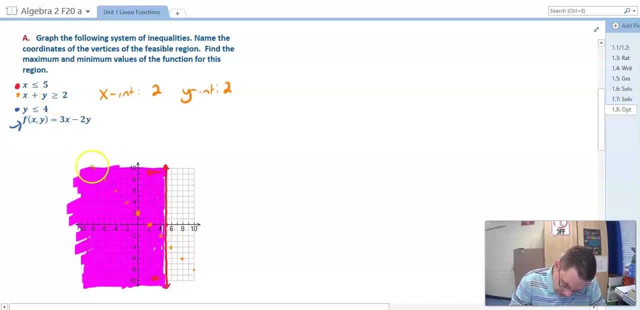 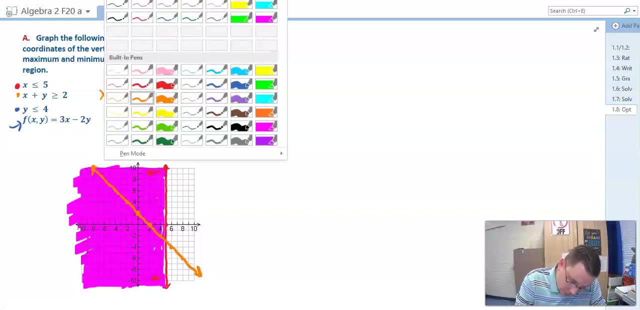 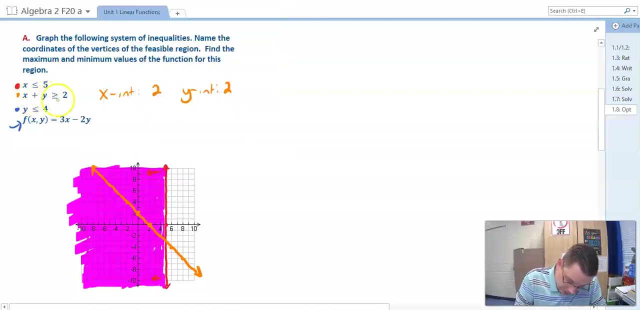 All the way up to the top. This line is also solid because it is equal to: and so I'm going to come all through here like so And so where is this orange shading going to be? Well, x is greater than or equal to x plus y is greater than or equal to 2.. So 0, 0 would. 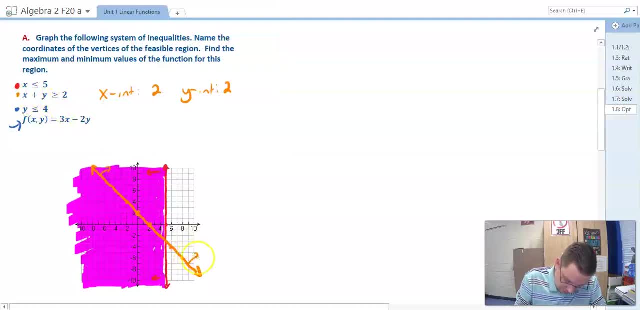 not fit here. so it's not going to be the origin, it's going to be this direction, And so my orange shading will be all of this. And again, we want to be as close and precise as possible, because we want to know where. 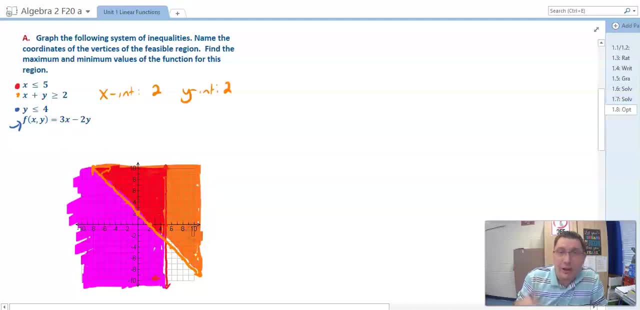 these intersections are going to be. This is the whole point of what we did in 1.7, finding those vertices. So the final one in blue, y is less than or equal to 4.. So y is 4, my line will go straight. 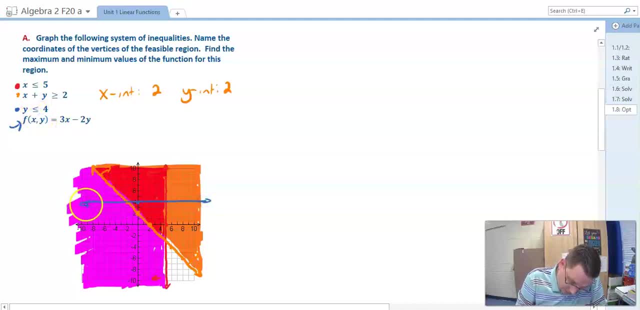 across at 4.. Less than or equal to means the shading will be below the line. And so where is my blue? It is all of this, And so where do the 3 overlap? And that is this little box right here I'm going to highlight. 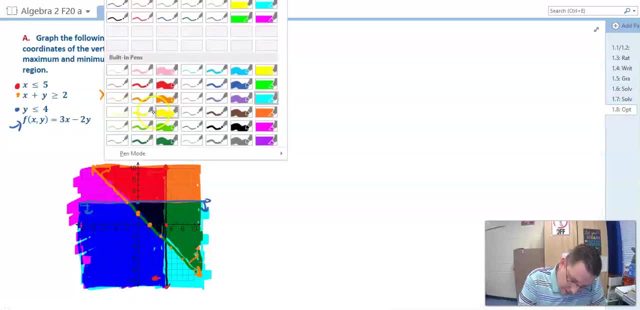 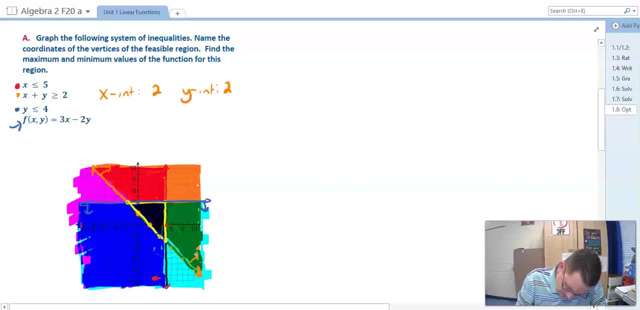 that in yellow, just to point it out a little bit better. All of this is our region. Now, the reason we did the vertices in 1.7 is for this next step. So let's list out our vertices into a table. So my first vertices is at negative 2 and then 1.7 in somewhere around there. Now here's the last problem. It's monitor. Maybe we'll check it later. Let's call the number into 10th place, if only So. I'm making this suit because theugh are going to help us. All the vertices are in the middle, Now where to? 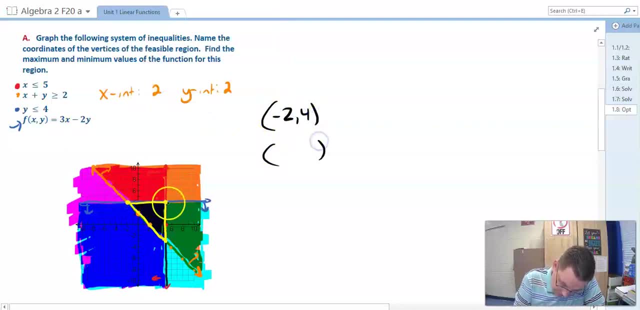 2, 4.. My second vertices is at 5, 4.. And my final vertices is at 5, negative 3.. Now look at that equation in the bottom. So we look at f of x, y is equal to 3x minus 2y. I want. 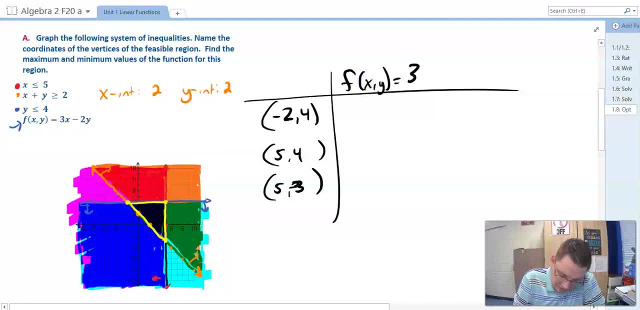 you to put that here in the table, Because what we're going to do- and this is the direction here- we want to find the maximum and minimum values of the function for this region, And so the maximums and minimums will only happen at vertices. Now there are occasions where 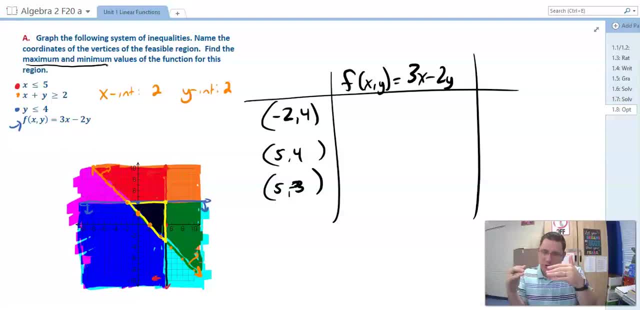 it will happen on a line because the maximum end goes along that whole line, But for the purpose of what we need to do, it's the vertices 98% of the time. So we're going to substitute this in. So we're going to get 3 times the negative: 2 minus 2 times the 4.. 3 times negative. 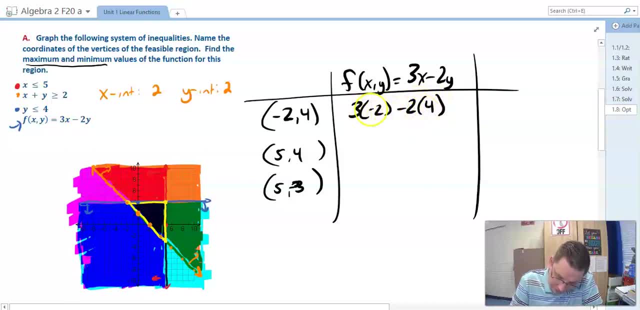 2 is negative 6.. 2 times 4 is 8.. So we get negative. 6 minus 8 is negative 14.. We do it for the second order pair, So 3 times the 5 minus 2 times the 4. So I've got 15 minus. 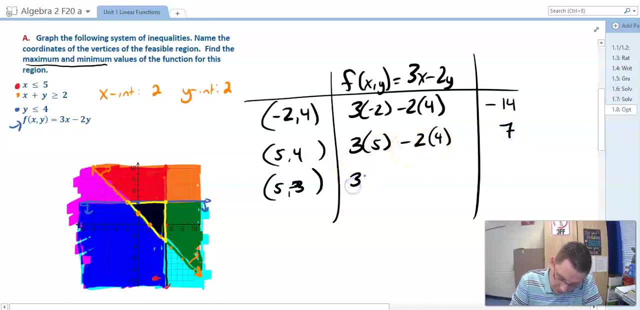 8 is 7.. And for the third order pair: 5 times 3,, 3 times 5, minus 2 times the 4. So I've got 2 times the negative 3. So that's going to be a positive 6 here plus 15 is 21.. And 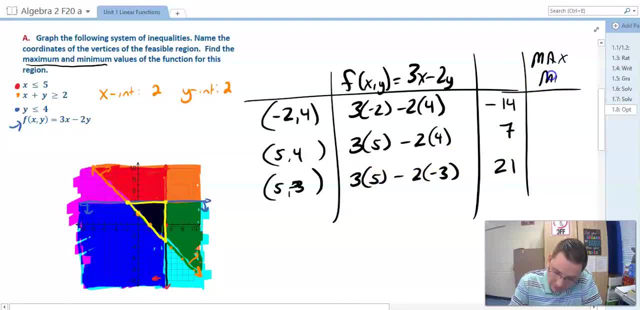 so when we look at these values, we want to know what is the max and what is the min, and where do they occur. Well, 21 is my max, So max, Negative. 14 is my min, So min. And where do they occur? So the max happens at 5, negative 3.. The minimum: happens at 5, negative 9.. And then we'll add up all the values to get the next one. So the maximal is at 5 minus 200.. So we're going to talk about how we can measure this f? f of 4, minus 5, minus 3, plus 5, negative 3, plus 5, minus 3.. And so we're going to 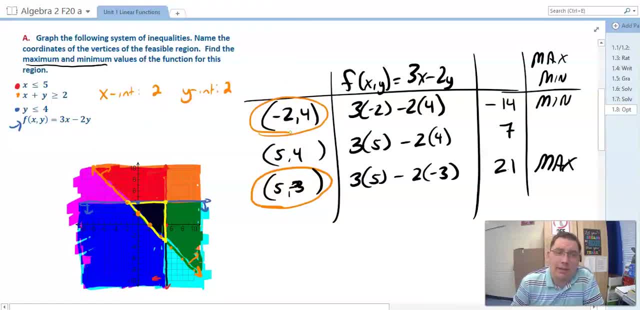 at negative, two, four. That's what we're talking about when we look at to maximize or minimize the value of a function. Now, this is just a graph on the coordinate plane, and we're going to look at a second example that's unbounded, and then we're going to have a word problem. we're going to look. 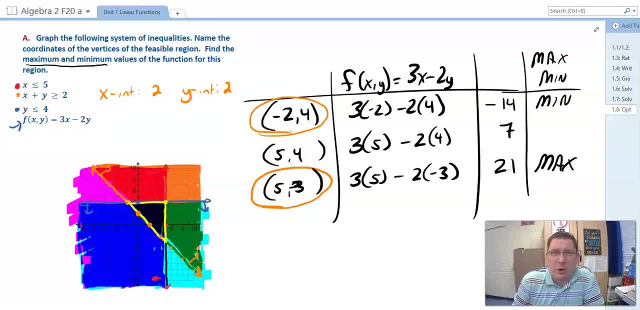 at where we want to know one end or the other. We're not always going to want to know both. We're going either to maximize, like our profits, or minimize our expenditures, and looking at those pairs will tell us that information. So here's example two, with an unbounded region. So it says: 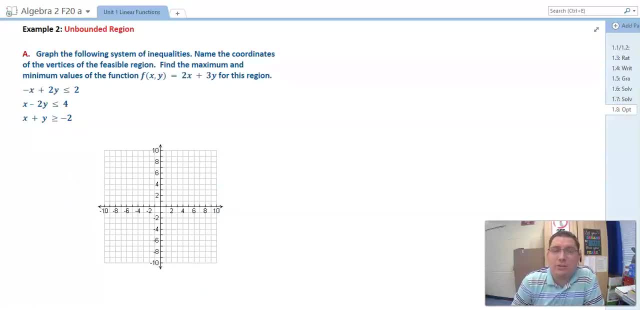 graph the following system of inequalities: Name the coordinates of the vertices of the feasible region and find the maximum and minimum values of the function f of x. y is equal to 2x plus 3y for the region. So they give us these three inequalities to graph, and so I want you to pause the video now. 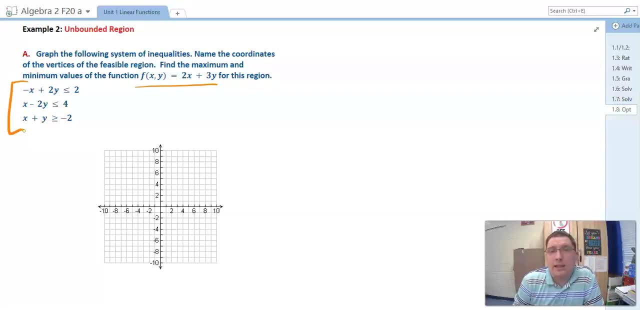 to graph these inequalities on the graph and then also find the vertices. So again, pause the video now, graph the inequalities and find their vertices and then come back. All right, so on the graph. here you see, I've graphed all three and I've listed out my x and y. 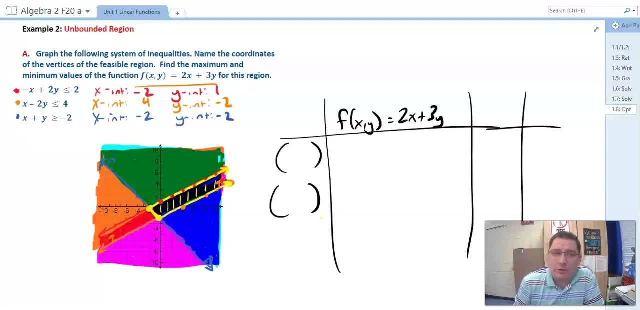 intercepts for all three. so if you've gotten a little confused on how to graph those or you need a review, I've got those listed there and again. if you've got questions on those, make sure you ask in class. But let's look at the vertices that this has. It only has two. The first one is here at the: 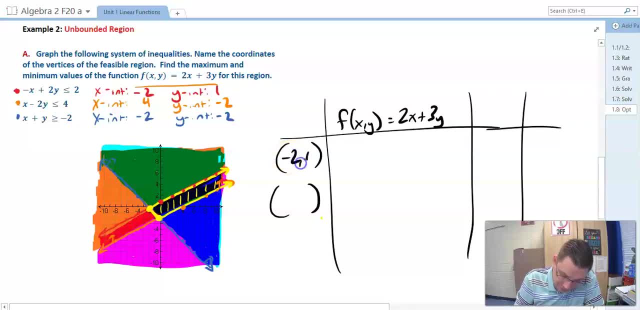 x- intercept of negative two, zero. The second one is this: y- intercept here of zero negative two. This is an unbounded region because that those two lines are parallel. they're never going to cross and create a closure of a third, and so this region goes on forever, But the max and mins will only be found at those. 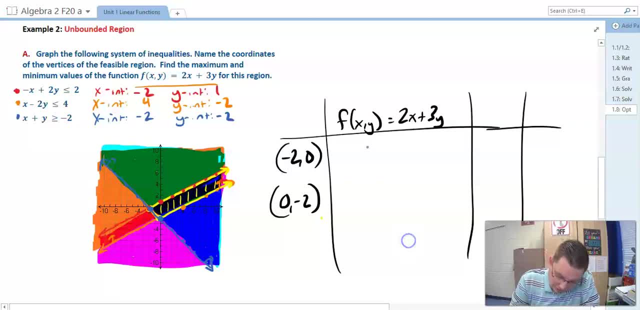 intercepts, And so let's talk about the values that we'll get here. So two times negative two plus three times zero, so that's negative. four plus zero is negative four. And two times zero plus three times negative two, that's negative six. because that's zero, that's negative six. So let's 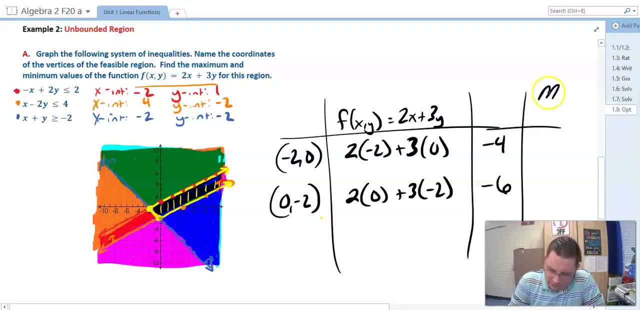 talk about what happens with this region, because we would normally list our maxes and our mins here. But the problem is, this is an unbounded region, and so you're only going to get one end or the other, And so let's think about this region. So let's think about this region. So let's think about this. 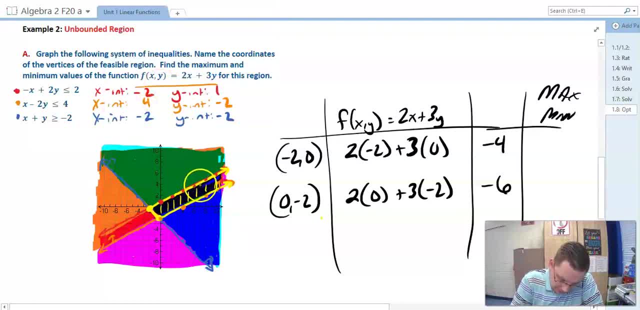 point that lies in the middle of this. So let's come and use like a point here: This is six four. So we'll do a third point here: Six four, And so we get two times the six plus three times the four. so 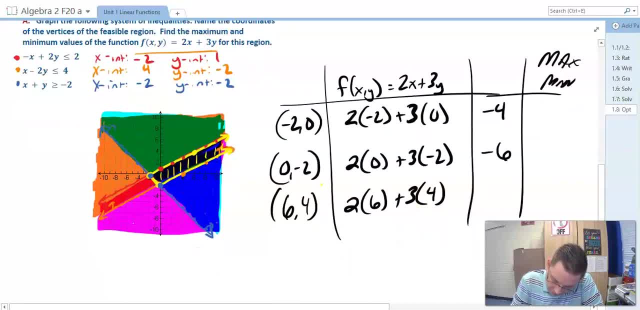 that's twelve plus twelve and that is twenty four. So that tells me that this is going to go into the positives, which means this negative four is neither, because it's not the smallest value, it's not the largest value And these values are going to continue to increase. 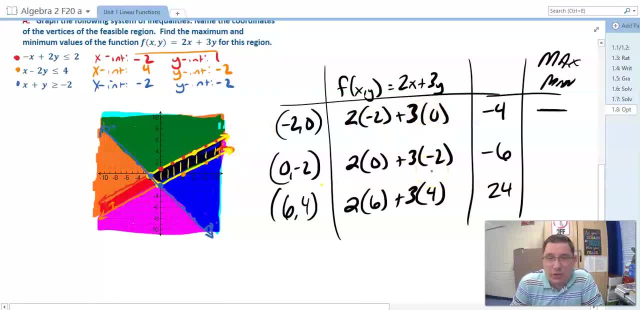 These are positive values multiplying to positives that have no negatives involved. This is going to increase And, remember, our vertices will determine either a minimum or a maximum, And so, because I have a value larger than what's going on, this will be my minimum. 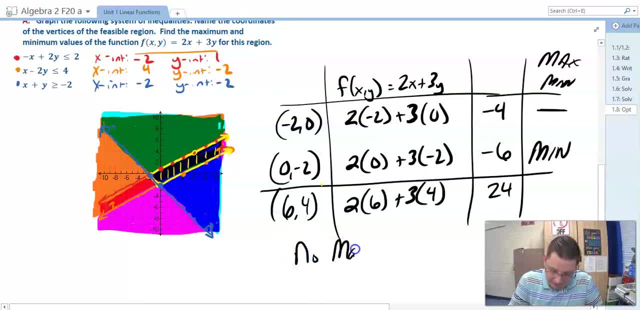 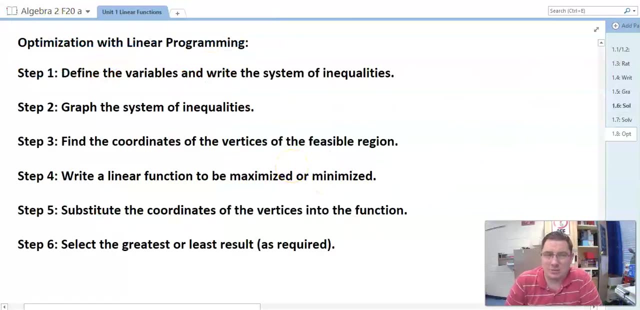 and I will have no maximum to this function because, again, it is an unbounded region. It will keep growing and growing forever and the values will keep going forever. So that's what we're looking at there, And so these are the six steps that it takes to deal with optimization, particularly in a word problem. 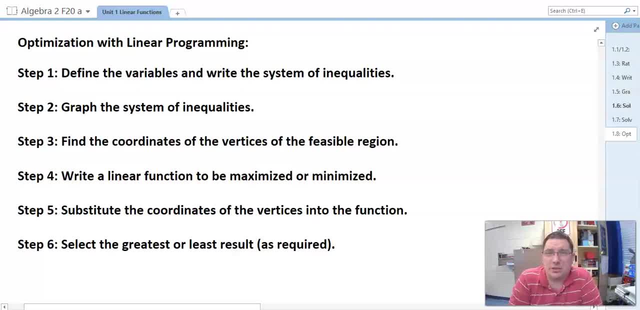 First, define the variables and write the system of inequalities. And so, as we look through the word problem, we're going to pick out the information that we need and we'll write our system. Step two: graph the system. Step three: find the coordinates of the vertices of the feasible region. 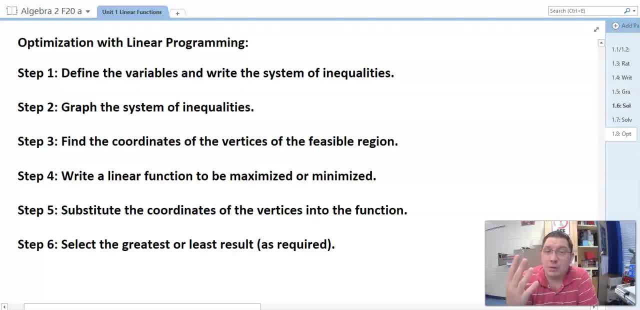 Step four: find a linear function. Step five: find a linear function to be maximized or minimized. Sometimes this is given to you immediately, Sometimes this is a part of the word problem. Step five: substitute the coordinates of the vertices into the function. 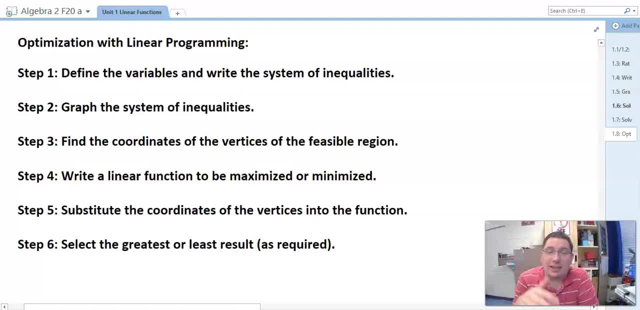 And step six, select the greatest or least result as required. So if we're trying to maximize something, we want the largest. If we want the least, then we're going to look for the minimum. So let's look at how this works in a word: problem. 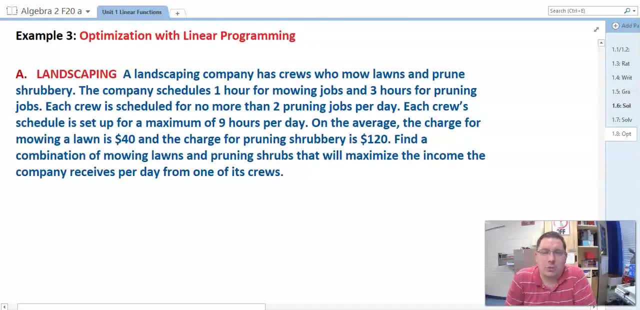 So the example is this: A landscaping company has crews who mow lawns and prune shrubbery. The company schedules one hour for mowing jobs and three hours for pruning jobs. Each crew is scheduled for no more than two pruning jobs each day. 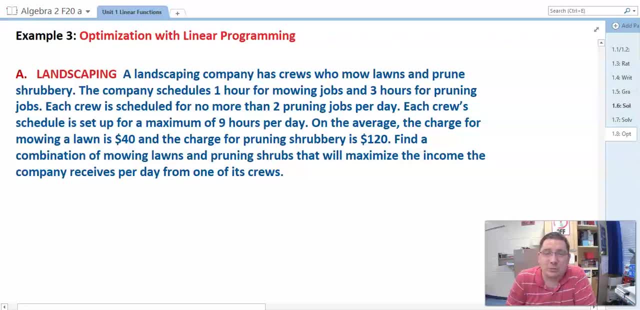 and each crew's schedule is set up for a maximum of nine hours per day. On the average, the charge for mowing a lawn is $40, and the charge for pruning shrubbery is $120.. Find a combination of mowing lawns and pruning shrubs. 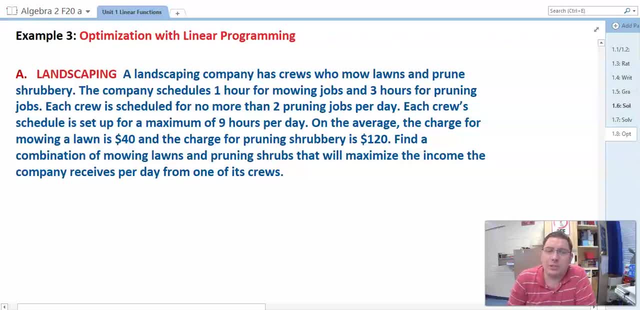 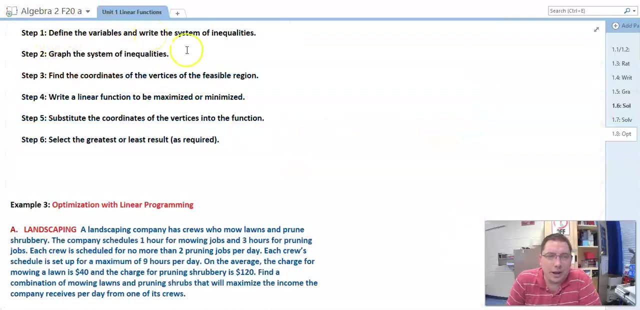 that will maximize the income the company receives per day from one of its crews. So let's review the steps. Step one says to define the variables and write the system of inequalities, And so when we look at this problem, our first variable in the problem is mowing jobs. 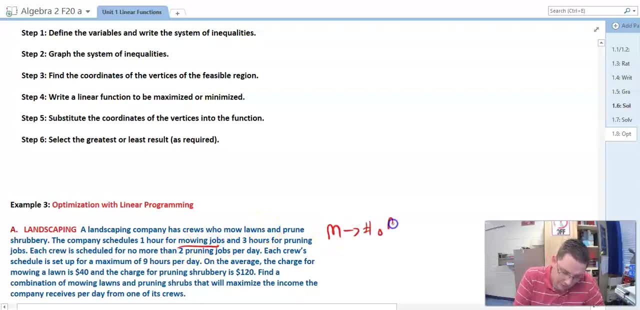 And so m will be the number of mowing jobs, And p will be the number of mowing jobs And p will be the number of pruning jobs. Now we need to write the system And we need to understand what information is going to come out of here. 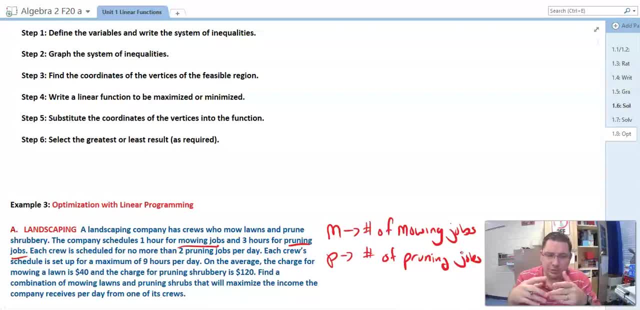 And so what are we trying to do here? We've got time involved and we've got cost involved, And so the cost is what we're trying to maximize. So that's going to be our function in the end, So that'll be the function that we build. 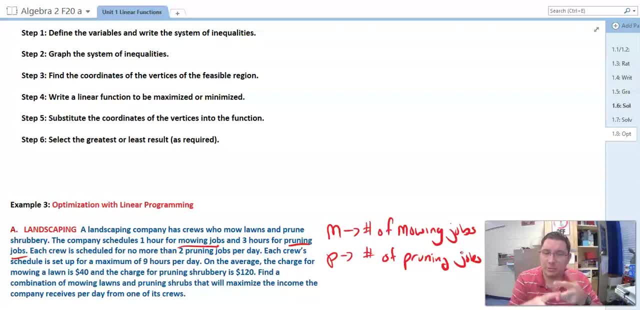 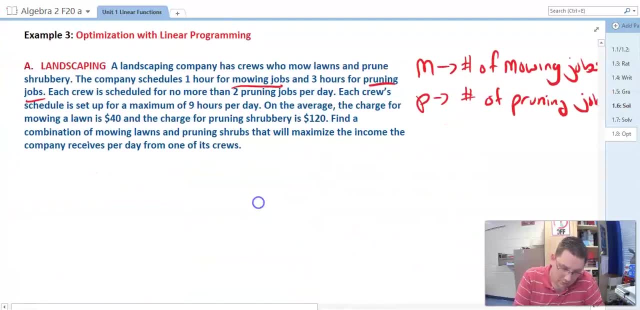 So what we're trying to deal with is how many mowing jobs and how many pruning jobs I can deal with, And so let's look at what those will be. Let's look at what those will be as we write the system. So we're told that each mowing job is one hour. 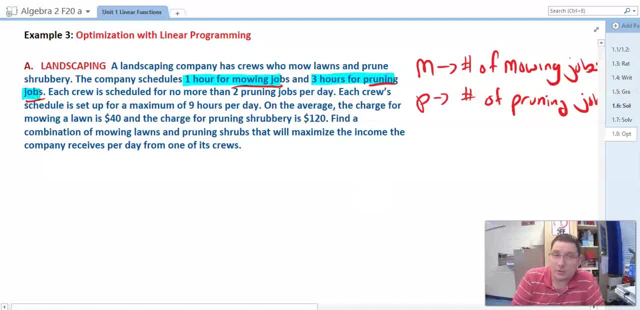 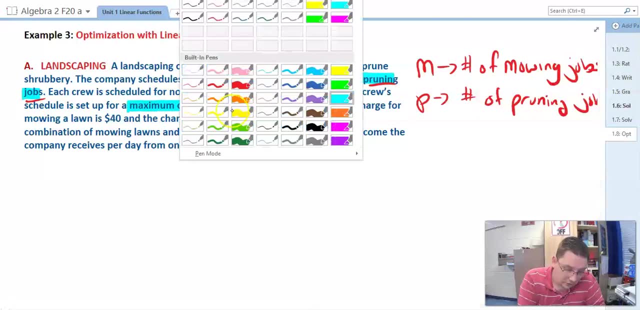 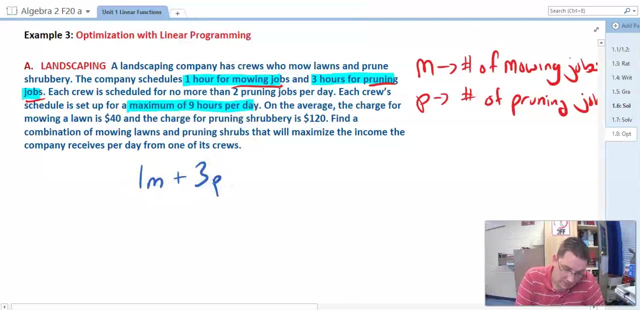 And we're told that each pruning job is three hours And they can work for a total of what? Nine hours per day. So as we build that up, we're going to get 1m plus 3p. maximum here has to be less than or equal. 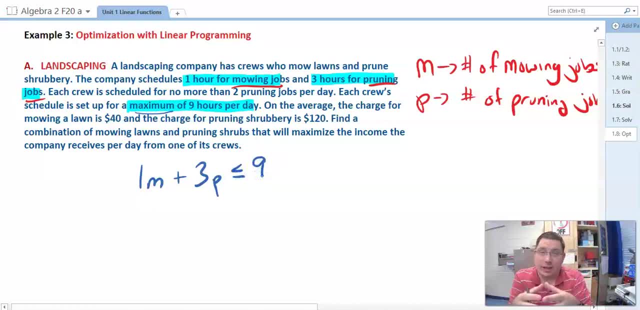 or equal to nine, because, again, our mowing jobs are an hour each, The pruning jobs are three hours each, And so, whatever combination of mowing and pruning that I do, that's what's going to come out to our time. Okay. 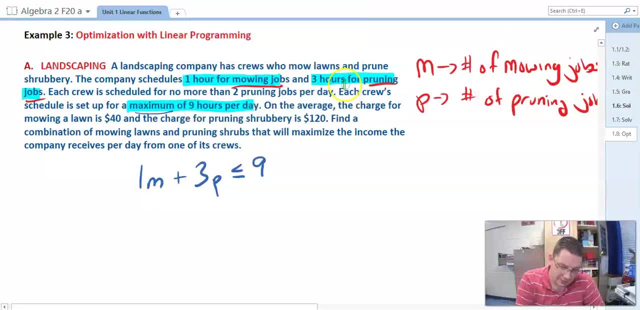 The second part here is this next sentence: It says that each crew is scheduled for no more than two pruning jobs per day, And so we have a second restriction here, that p the number of pruning jobs that I do must be less than. 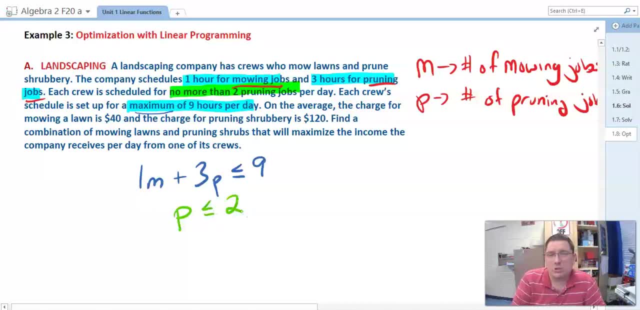 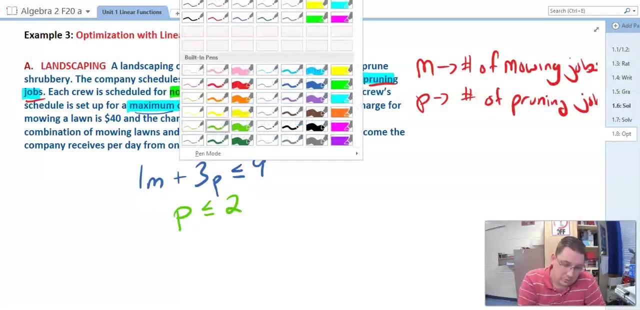 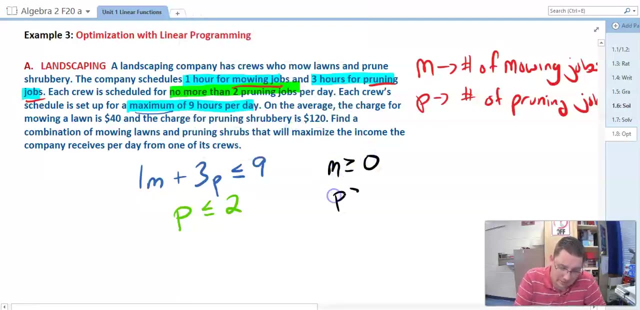 or equal to two, And so those are the two inequalities we're going to deal with in this situation. Now, obviously, we are restricted to the first quadrant, And so two other constraints that we would have here is that m, of course, has to be greater than or equal to zero, and p has to be greater than or equal to zero. 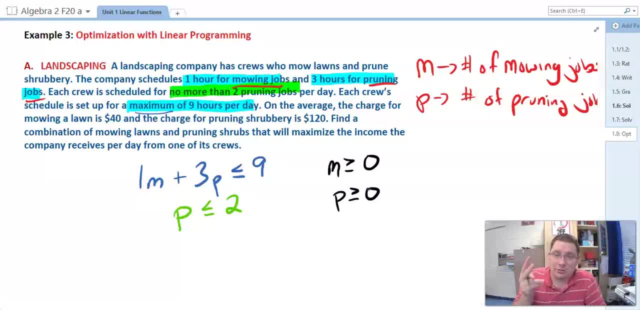 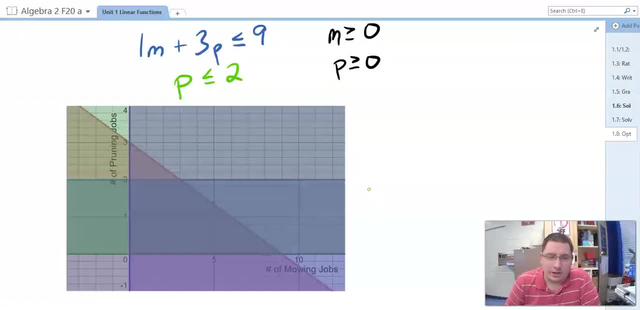 And so let's see what that graph is going to look like, because that is step two. What is our graph? So, as you see, here I've graphed up the inequalities that we have, And so, just to give you an idea of which one's which this one coming here is the one: m plus three p is less than or equal to nine. 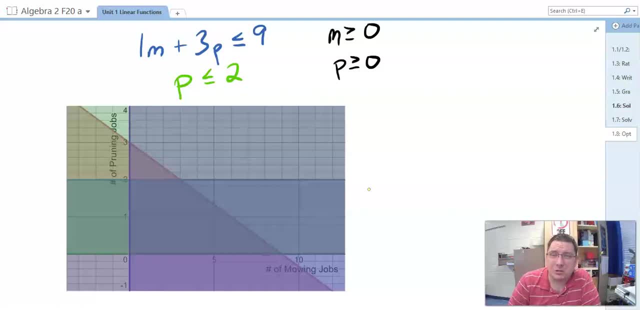 The horizontal one here is the p is less than or equal to two, And you also see that I have that m is greater than or equal to zero and p is greater than or equal to zero. So where do all these overlap? It's going to be the darkest shading that we have. 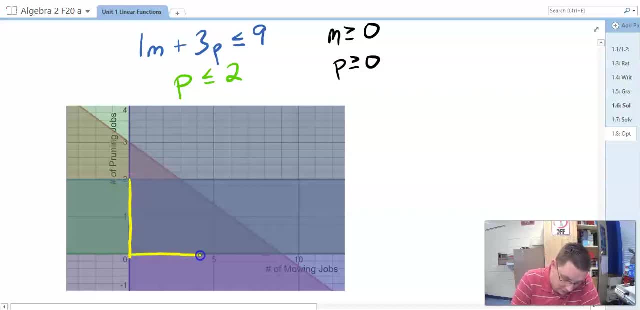 And so it creates this trapezoidal figure here. And, as we talked in the first half of this lesson, we talked about where the maximums or minimums can happen, And so we want to look at the vertices, And so I've got one. 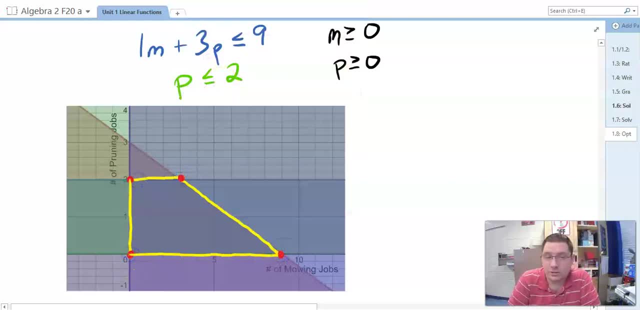 two, three, four vertices to deal with, And so we want to label all those out, And so I've got zero, zero, zero, two. This is three, two, and then over here is nine, zero. And, like we did before, 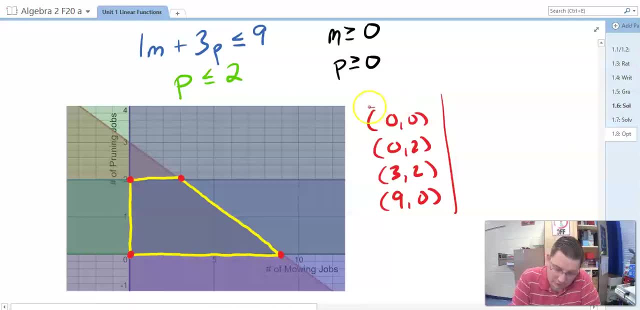 our next step is to deal with our function. right, So we're going to set up our table and have some function here- F of m, p, but we haven't written our function yet, So let's go back to the word problem. 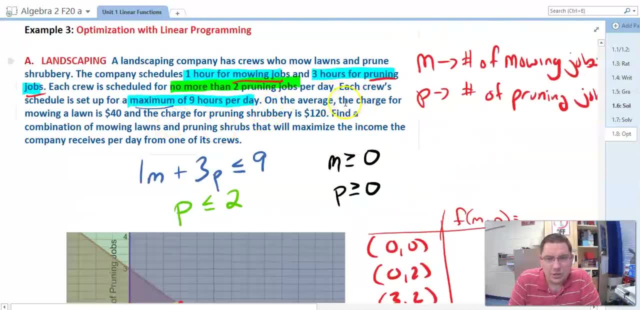 When we look at this word problem, it says: on average, the charge for mowing a lawn is $40 and the charge for pruning a shrubbery is 120.. So this is what's going to build our function. F of m. p is equal to what? 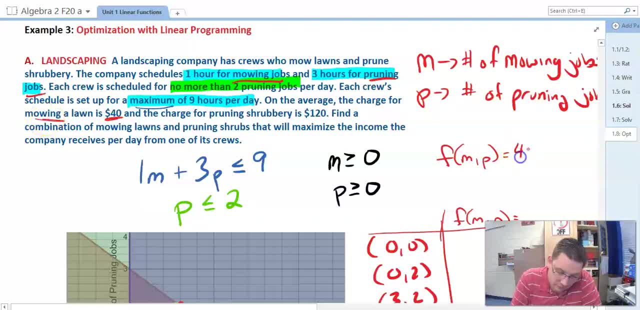 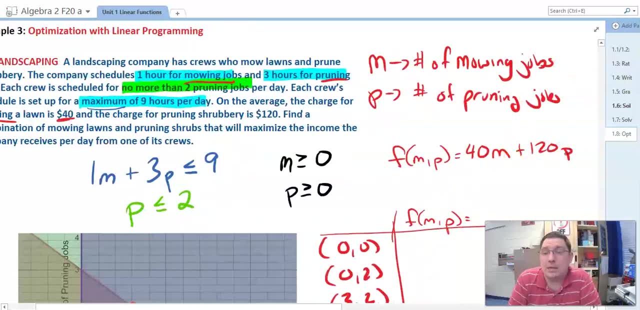 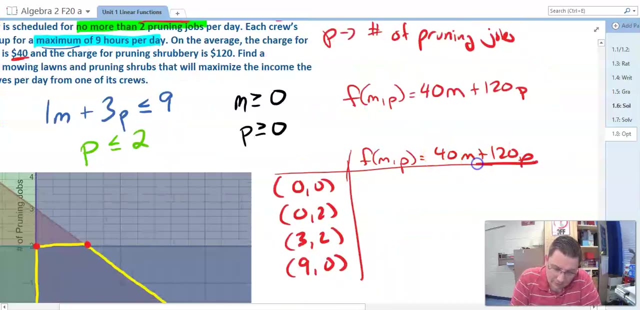 Well, for each lawn they mow, it is $40.. So 40 times m, and then, for each pruning job, 120 times p. Now, that's what we're going to put here, And so we're going to try it for each one. 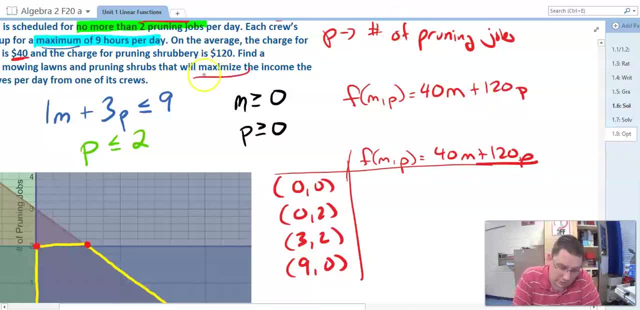 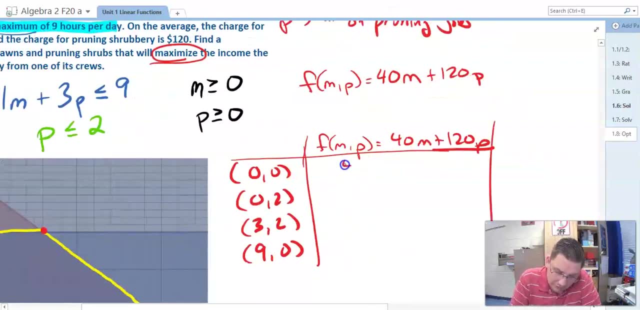 figure out which is our max, Because that's what we're trying to get here, right? We're trying to maximize the income. I don't care about the minimum in this problem, Okay, And so we plug it in for each. So zero plus 120 times the zero. 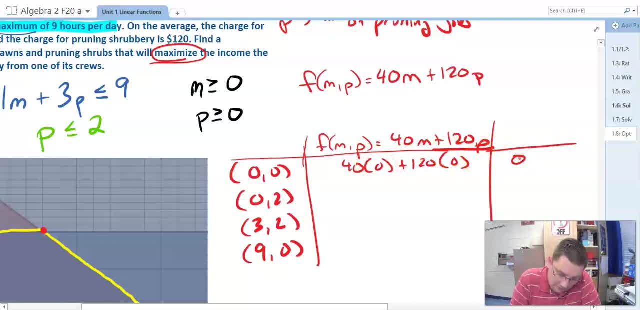 That is going to give me zero, because zero plus zero is zero. And then here I've got 40 times the zero plus 120 times the two, So it's gonna be 240. here I've got 40 times the three and 120 times the two. 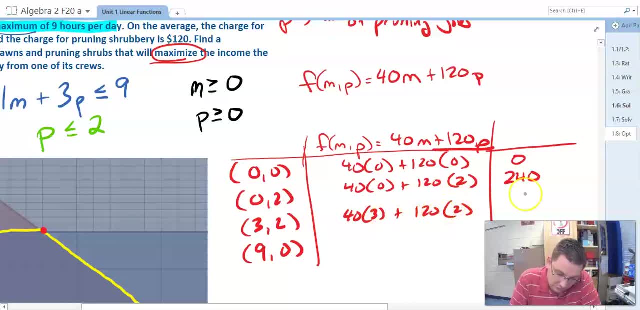 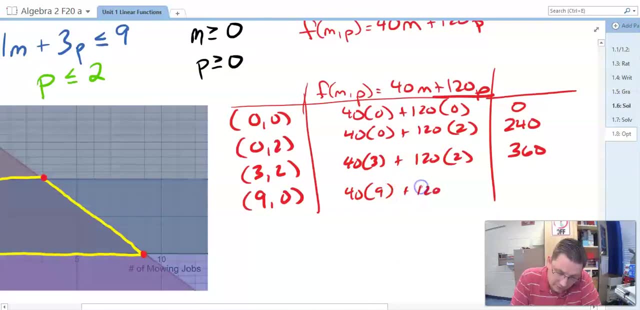 So 40 times three is 120.. This is 240.. So it gives me a total of 360.. And then finally here, 40 times the nine plus 120 times the zero, That'll also give me 360.. And so again, 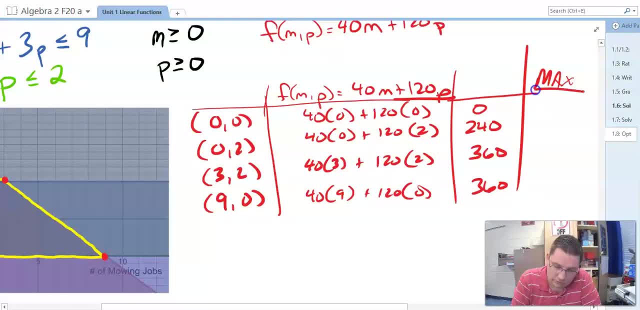 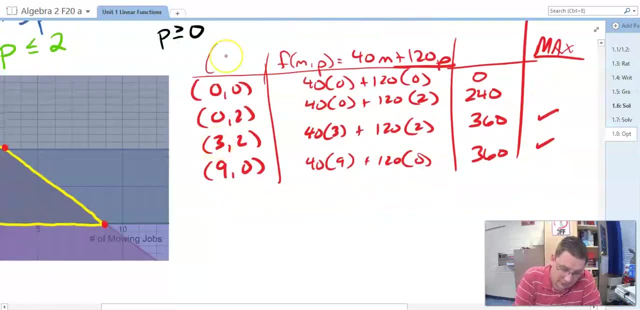 I'm looking for the maximums, So where's my maximum? I actually have two here that I could do, What? Well, remember that the first is m and the second is p. So I could do. I could do three mowing jobs and two pruning jobs. to earn how much? 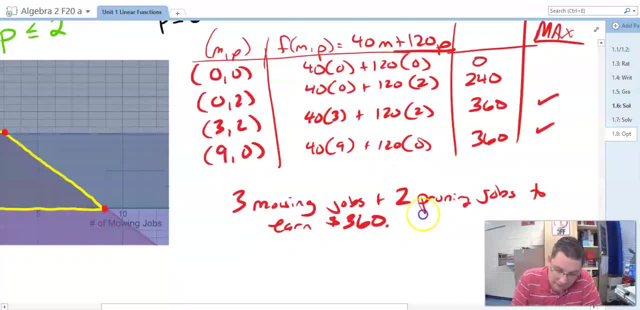 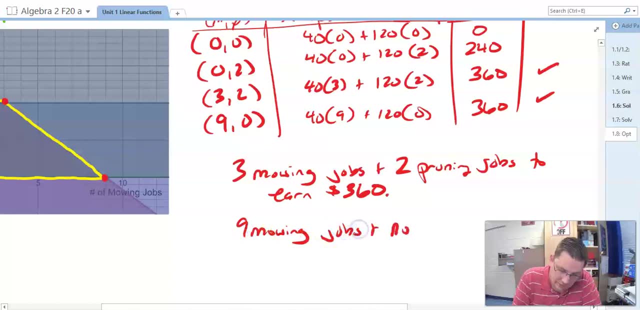 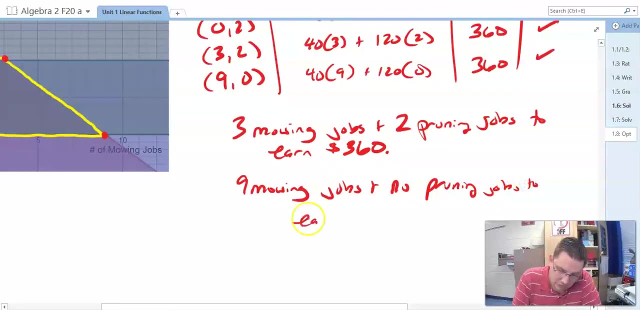 $360.. But I could also do nine mowing jobs and no pruning jobs. So here in this problem it gives me two. so I could do nine mowing jobs and two pruning jobs to earn $360.. So in this problem 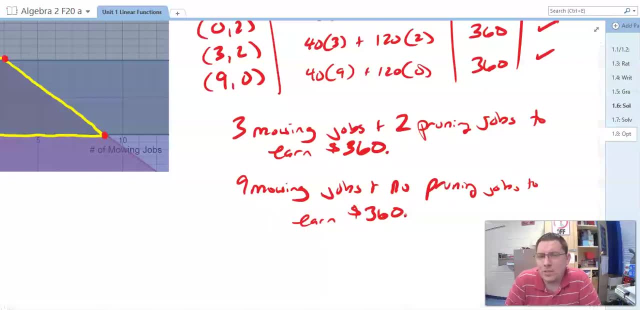 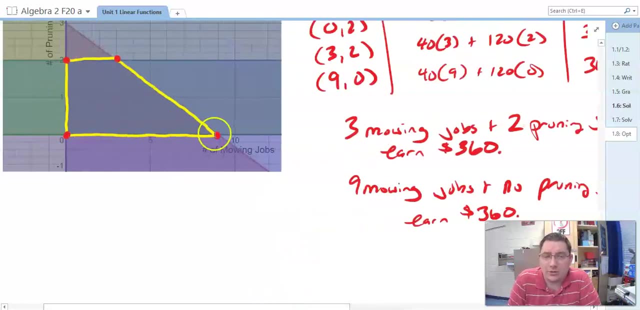 we see that this actually has two maximums that we can work with here And remember: maxims and minims will only occur where At our vertices, And so either one of these two answers is acceptable for the final answer. You don't necessarily have to find both. 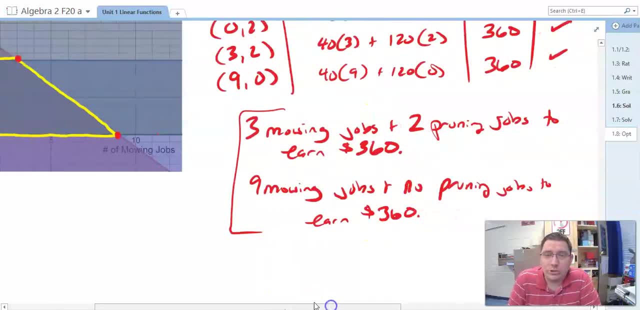 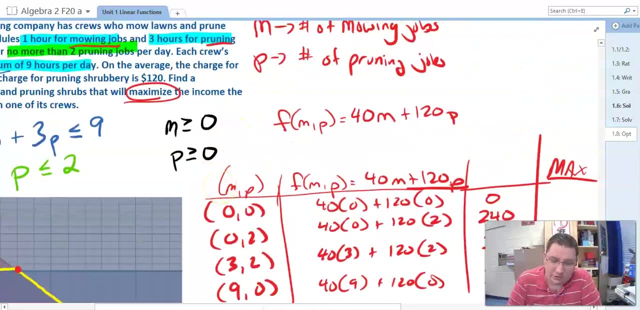 but you do need one or the other. Now, what would change this problem? Let's just talk hypothetical first for a second. what would change this problem? well, couple things could change it, right? let's say there's no restriction on the pruning jobs, right? so 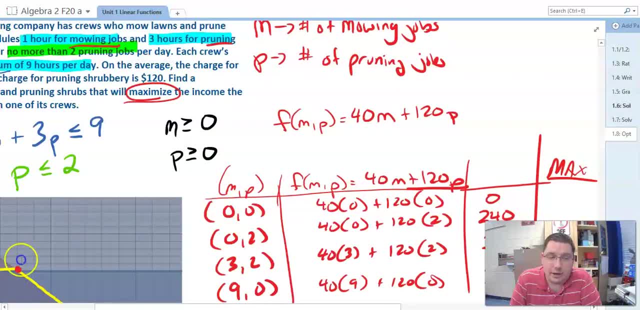 that would change this line and I would not have a maximum occurring here anymore. or I could change how much pruning jobs and mowing jobs are. maybe mowing jobs are worth $50 each and pruning shrubbery is 125. that would change where our max would occur and so, again, that is a possibility in these. 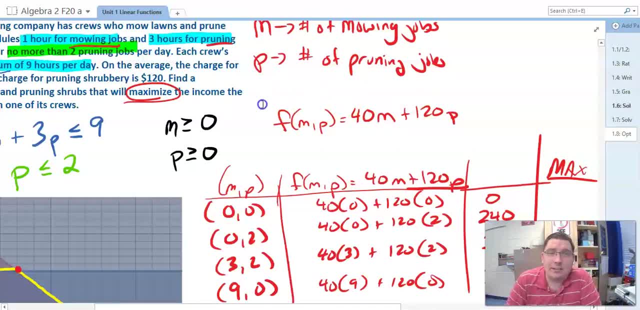 problems. okay, so that's it for today. that ends this unit on unit one on linear functions, and so we are going to be preparing for the unit test. so be looking out for the unit review video and then be preparing for your tests, and I hope you all have a good one and see you next time.